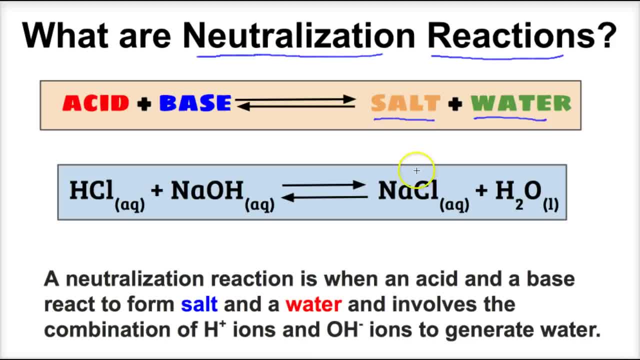 Now you might be thinking of salt as the sodium chloride or the table salt that you put on your dinner. However, in chemistry, a salt is any ionic compound Or any compound where you have a positive ion bonded to a negative ion, For example. we have dozens and dozens of different types of salts in chemistry. 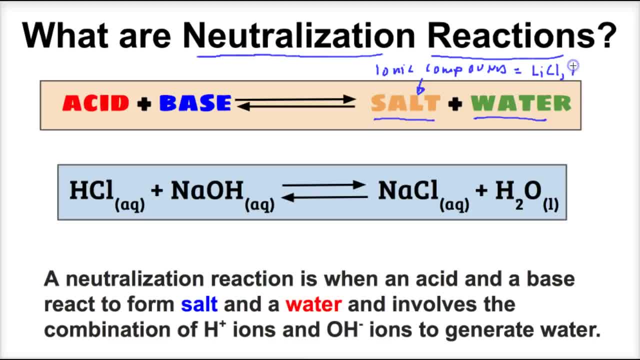 We've got lithium chloride. there is a salt. We've got ammonium nitrate. that would be another example of a salt. Alright, so a salt in chemistry is anytime you have a positive ion bonded to a negative ion or an ionic compound. 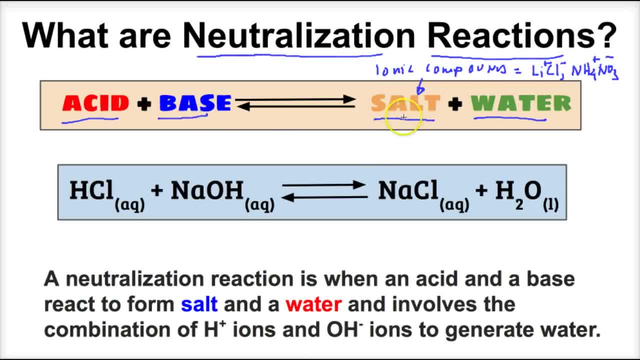 And anytime you have an acid And you react it with a base and it produces a salt and water, you will have what is called a neutralization reaction. And here's what's happening, people Right here we have hydrochloric acid reacting with sodium hydroxide. 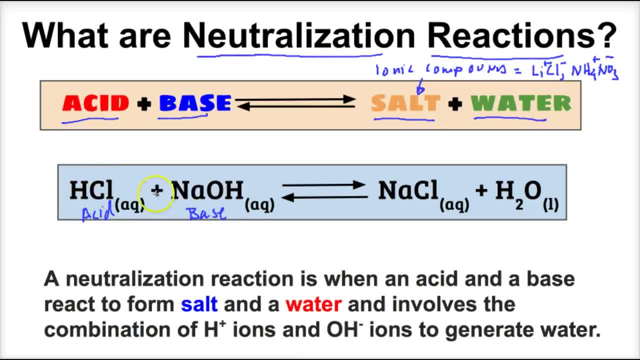 You can tell this is an acid because acids typically start with hydrogen, And you can tell that this is a base because bases typically end in OH or hydroxide. Okay, So this is an acid, because it starts with H usually And this is going to be a base. 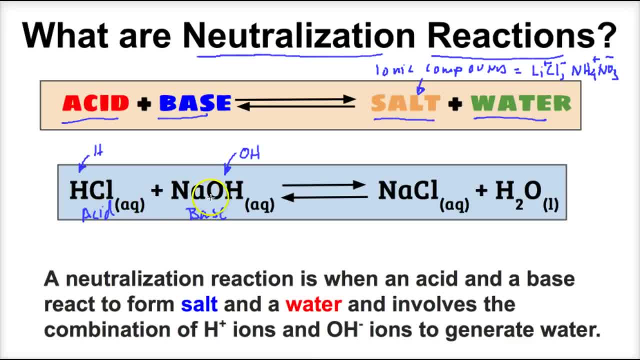 And this is going to be a base, because it ends in OH And anytime you have an acid reacting with a base and it produces salt and water, you have a neutralization reaction. But here's what's happening, people. What ends up happening is that the hydrogen from the acid is going to bond with your OH from the base to produce your water over here. 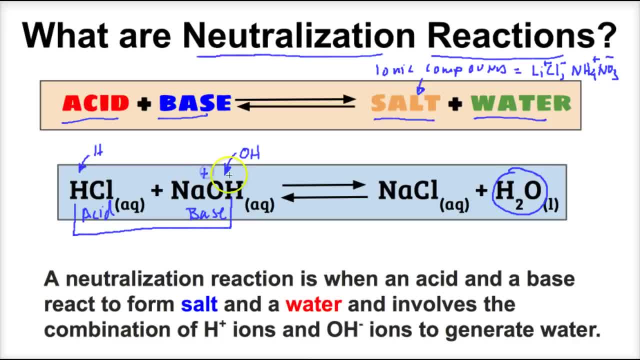 And then what ends up happening is the positive ion from the base. remember that sodium is a positive one and hydroxide is a negative one, And that chloride is a negative one And that sodium is a negative ion over here. So what ends up happening is that the positive ion from the base is going to end up bonding with the negative ion from the acid to produce your salt over here. 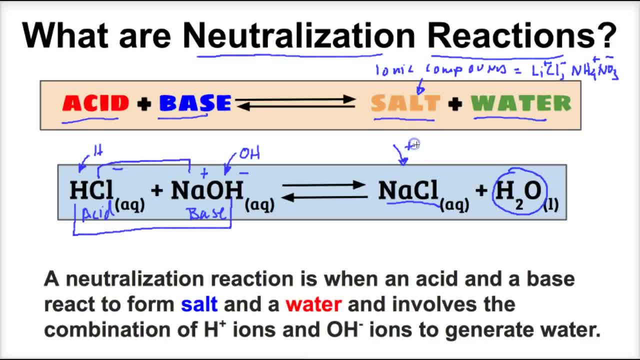 And when we write the chemical formula for this salt here, always remember that the positive ion comes first when you're writing the chemical form or symbols, followed by the negative. All right, So it's not ClNa, It's going to be NaCl for your salt over here. 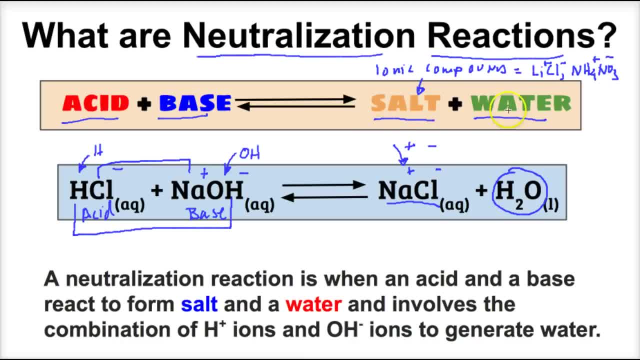 All right. So, once again, whenever you have an acid and a base and salt and water is produced, you have a neutralization reaction And what ends up happening is that the hydrogen from the acid is going to bond with the OH from the base to produce your water over here. 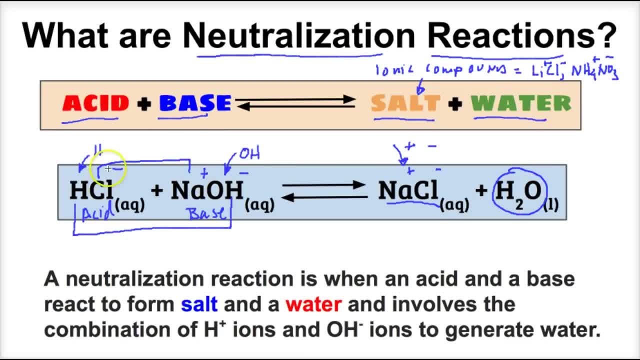 And then the positive ion from the base is going to bond with the negative ion from the acid to produce your salt over here. Okay, So knowing this, what we can do is we can predict what the products of a chemical reaction will be. So let's take a look at a couple of examples. 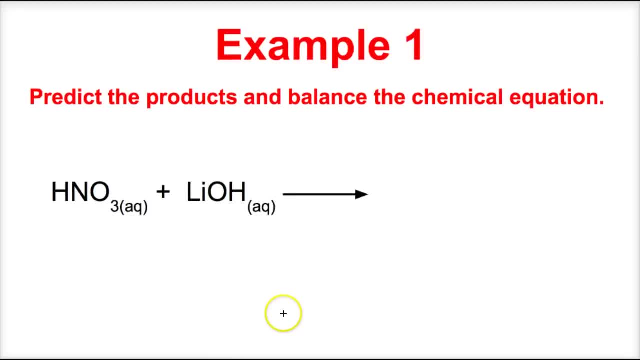 Okay, So in this example here it says to predict the products and balance the chemical equation. So if we take a look at this, we have an acid here. This is nitric acid And we learned how to name acids earlier in the year. 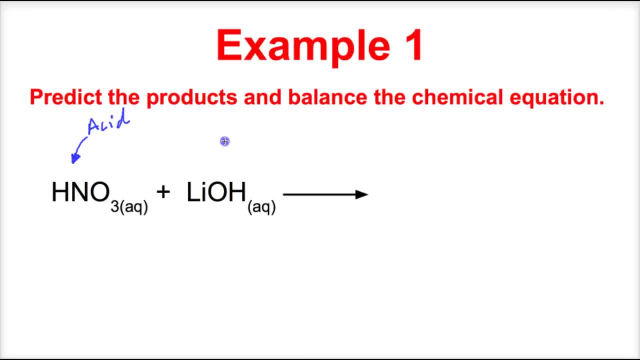 So we have an acid here And we have a base right here, And you can typically tell that this is a base because it ends in OH. Okay, So we just got them saying that whenever you have an acid and a base that ends in OH like this, what ends up happening is that the acid is going to bond with the OH. 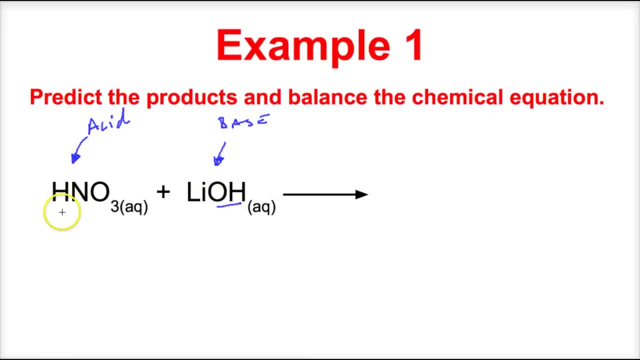 Okay. So whenever you have an acid and a base that ends in OH, like this, what ends up happening is that the acid or the hydrogen from the acid is going to bond with the OH from the base to produce your water or H2O in the liquid state. 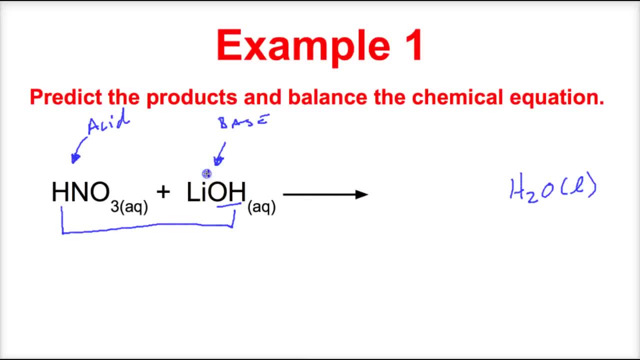 And then what happens is that the positive ion from the base- remember that lithium is a positive one ion and hydroxide is a negative one, And that nitrate is a negative ion- here, negative one ion. So the positive ion from the base is going to bond with the negative ion from the base. 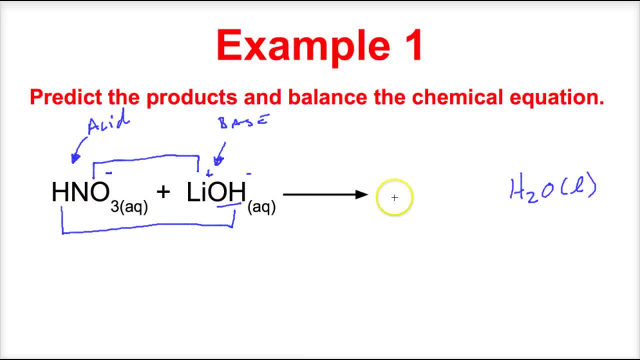 And that nitrate is going to bond with the negative ion from the acid to produce your salt. So what will the salt end up being? Well, is it going to be NO3LI Or is it going to be LINO3? Remember, the positive ion always gets listed first. 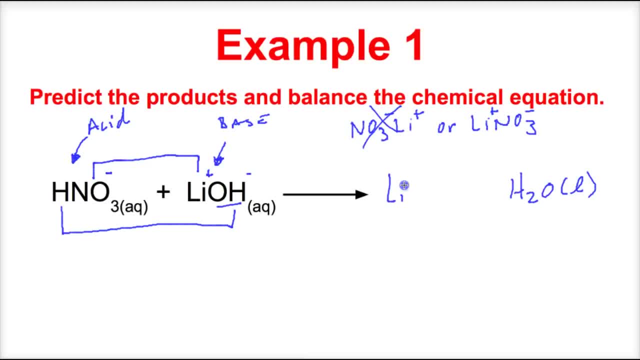 So this would be incorrect And it's LINO3.. Now, keep in mind, we need to make sure that these ionic charges add up to zero. So we have a one plus lithium ion And a one minus nitrate ion And, yeah, those add up to zero. 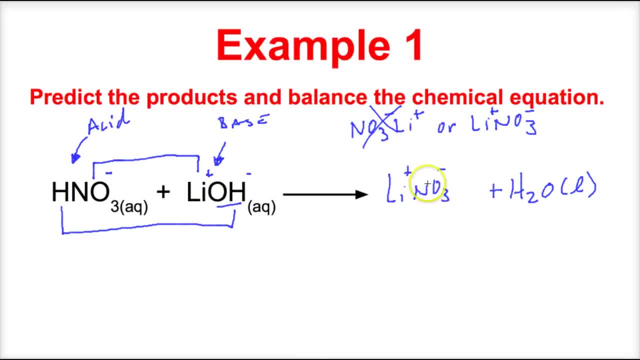 So you don't need to add any subscripts to this chemical compound here. And if you look at a solubility table on Google, you'll find that lithium nitrate is dissolvable in water, So we'll put in AQ. Alright, so we predicted the products. 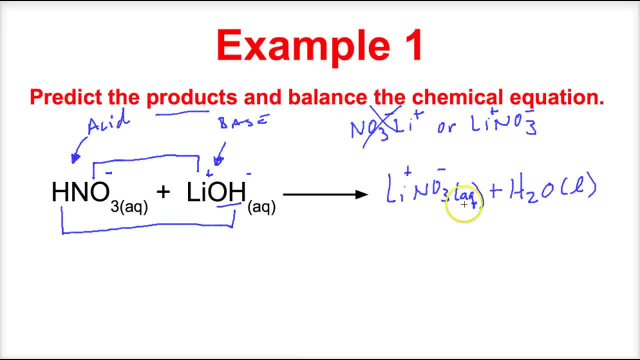 The products of this chemical reaction are going to be lithium nitrate dissolved in water and liquid water. So this is our salt And this is our water, right here. And whenever we have an acid in a base, it produces salt and water in a neutralization reaction. 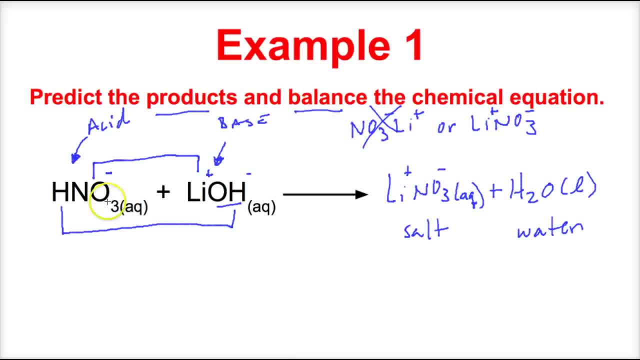 Alright. last thing, it says to balance the chemical equation. So if we take a look, this chemical equation is in fact balanced. If we take a look, we have one hydrogen, two hydrogens on the left, We have two hydrogens on the right. 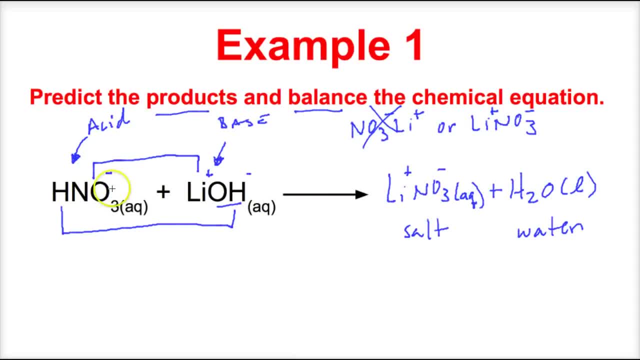 We've got one nitrogen on the left, one nitrogen on the right. We have three oxygens here, plus this one right here is four oxygens. We have three here plus the one right here is four oxygens. We have one lithium on the left, one lithium on the right. 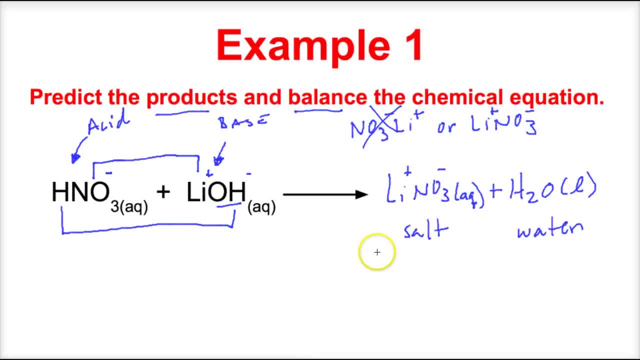 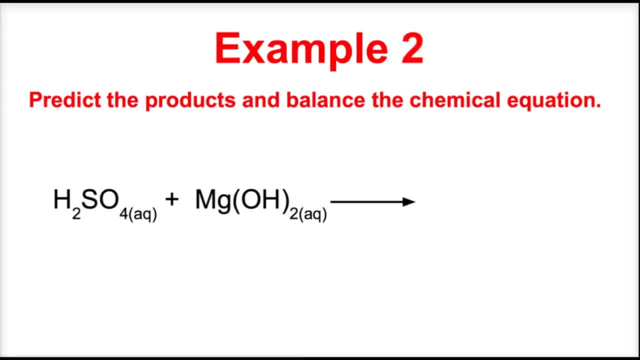 So we've predicted the products and we've balanced the chemical equation. There we go. Let's take a look at another example. Alright, so in this example here we have H2SO4, which is sulfuric acid, So we have an acid here. 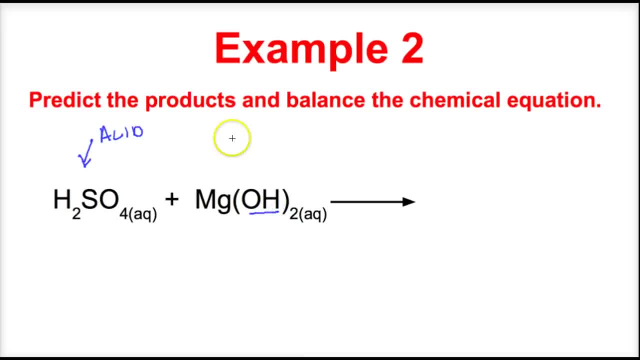 And we have magnesium hydroxide. This ends in hydroxide. That's a good indication that that substance will usually be a base. So we have an acid-base reaction And what we have to do is predict the products and balance the chemical equation. 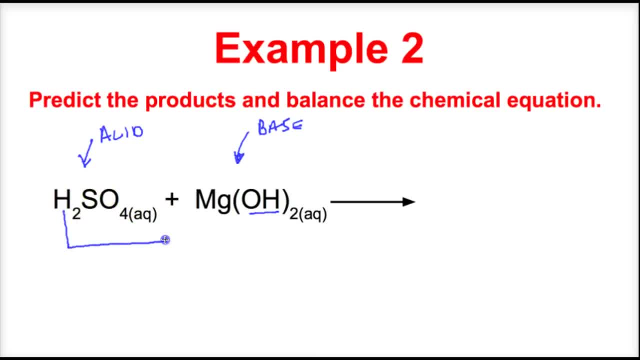 So, once again, what ends up happening is that the hydrogen from the acid is going to bond with the OH from the base. In fact, what ends up happening is that sulfuric acid is a diprotic acid. It's going to actually donate two hydrogens. 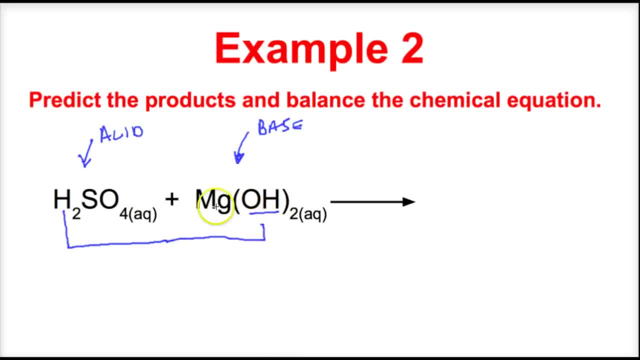 But that doesn't have any issue or bearing on this type of problem here. So what ends up happening is that the hydrogen from the acid is going to bond with the OH from the base to produce your water, your liquid water, over here, And what else is going to be produced. 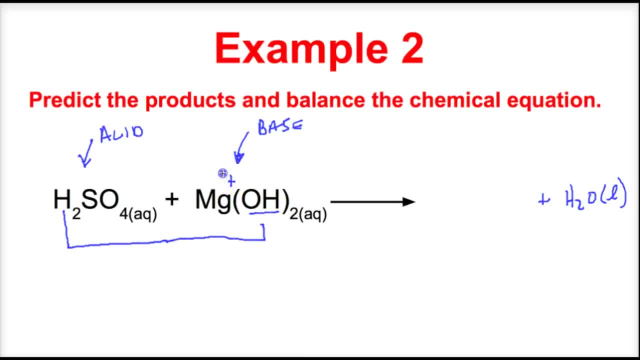 Well, the positive ion from the base- remember that magnesium is a 2 plus ion- is going to bond with the negative ion from the acid. remember that sulfate is a minus 2 or 2 minus ion and that's going to produce your salt. 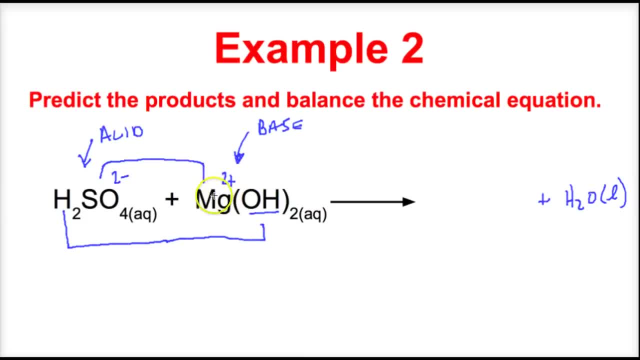 And when we write this, we always write the positive ion first, followed by the negative ion. So we have magnesium, Which is a 2 plus ion, And sulfate, which is a 2 minus ion, And because these two ionic charges add up to zero, 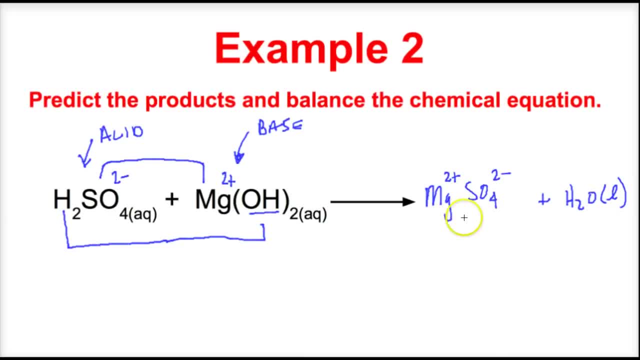 we won't need to add any subscripts down here. So MgSO4 is the correct chemical formula And, lastly, if you look at a solubility table, you will see that this is dissolvable or soluble in water, And so therefore it's aqueous. 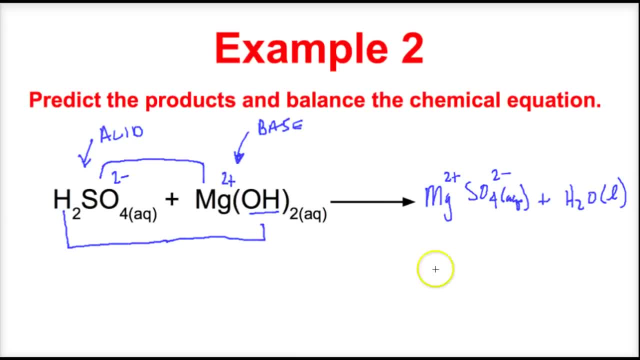 So there are the two products. Last, what we need to do is balance the chemical equation, And it looks like if we simply put a 2 right here, our chemical equation is now going to be balanced right. We've got 2 hydrogens on the left. 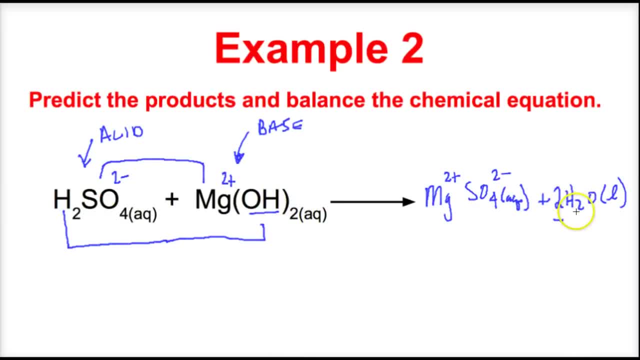 plus these two, here is 4 hydrogens on the left. 2 times 2 is 4 hydrogens on the right. We've got 1 sulfur on the left, 1 sulfur on the right. We have 1 magnesium on the left, 1 on the right. 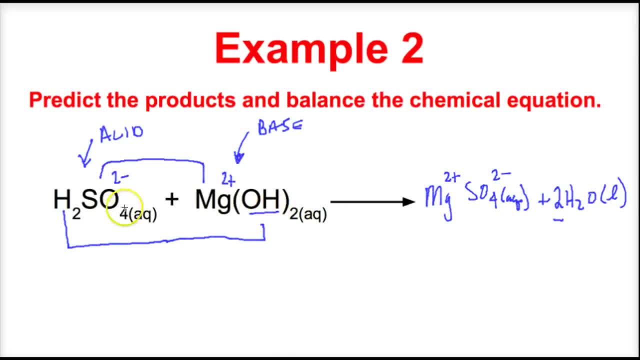 And it looks like we've got 2 oxygens here plus these 4. here is 6 oxygens. on the left, 4 oxygens and the 2 right. here is 6 oxygens on the right. So now you have a balanced chemical equation. 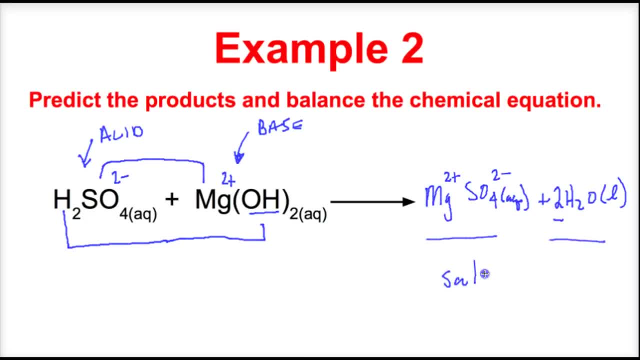 and you've predicted the products. So the magnesium sulfate here will be your salt and it looks like the H2O, of course, is going to be your water. All right, so let's take a look at another example. Okay, in this final example we have nitric acid. 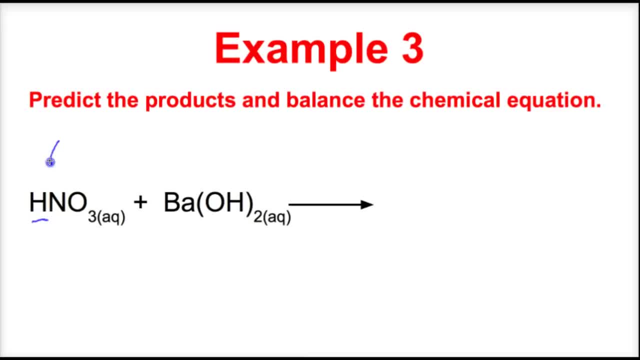 And we can typically tell this is an acid because it starts with H, so we have nitric acid. This is an acid And it's reacting with barium hydroxide. We can tell this is a base because it ends in OH. 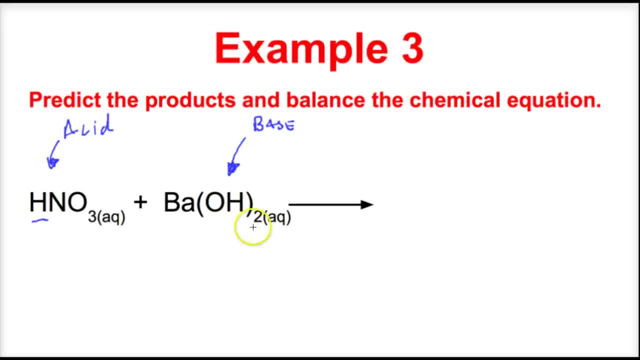 and usually that's going to be a base in organic chemistry. All right. so whenever we have an acid in a base like this, what ends up happening is that the hydrogen from the acid is going to bond with the OH from the base to produce your liquid water over here. 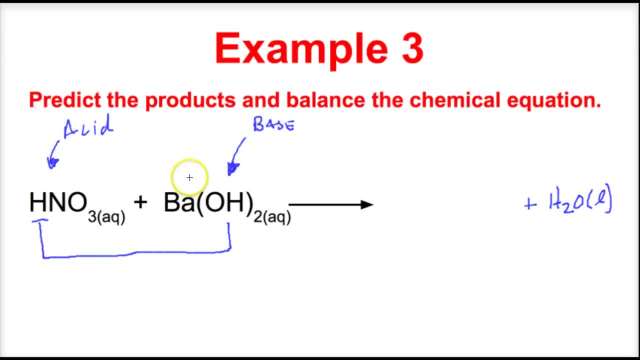 And then what happens is that the positive ion from the base- remember that barium is a 2-plus ion- is going to bond with the negative ion from the acid- Remember that nitrate is a 1-minus ion. So these two guys are going to bond. 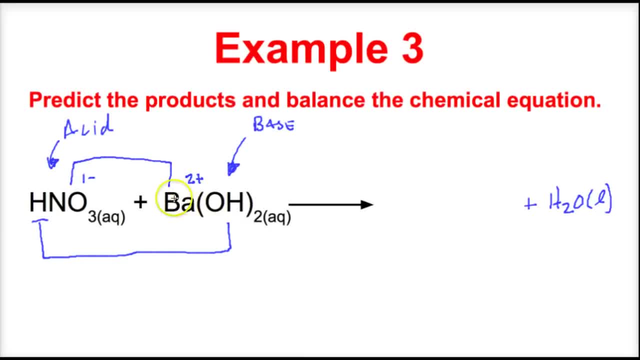 and join together. And when we write the chemical formulas, the positive ion always comes first. So barium, which is a 2-plus ion, and nitrate, which is an NO3, 1-minus, or just simply we'll just put minus right here. 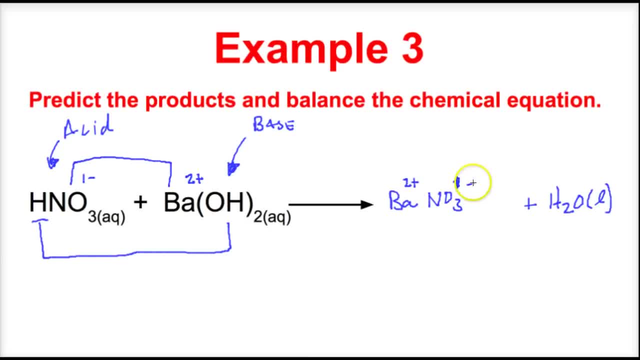 All right. so when you're writing the chemical formulas, the ionic charges don't need to be here, but what you do need to have is the correct subscript. So these two ionic charges do not add up to 0 right now. 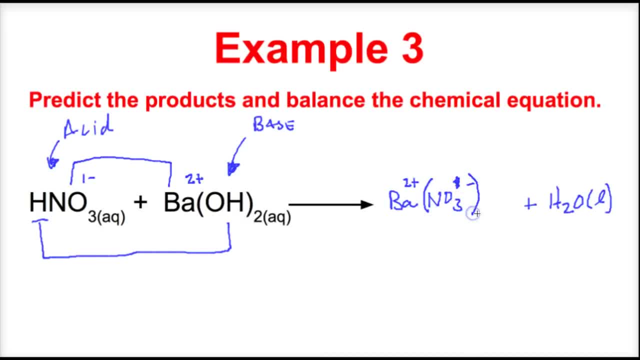 And in an earlier video we learned that you're going to have to put parentheses around this and then put a 2.. And then, if you look at the solubility table, you'll see that barium nitrate is soluble in water. 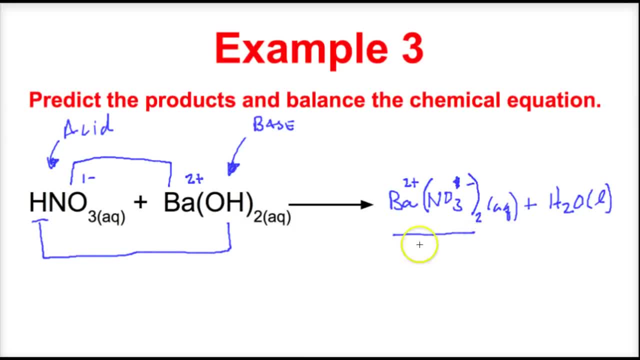 So there we go. We just predicted the two products. We have our salt, which is going to be the barium nitrate, and we have our water over here, And the last thing that we will have to do is balance the chemical equation. 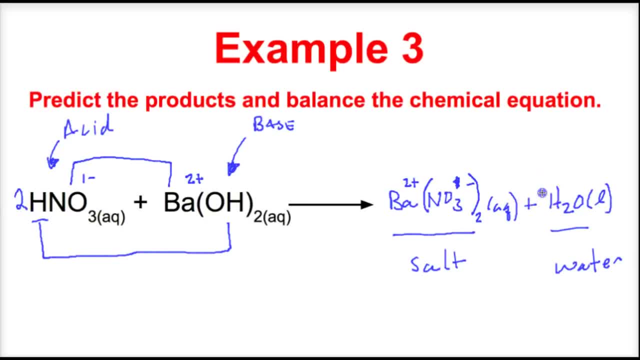 And if I put a 2 right here and then put a 2 right here, our chemical equation should be balanced. Let's check it out. We have 2 hydrogens here plus the 2 here is 4 hydrogens on the left. 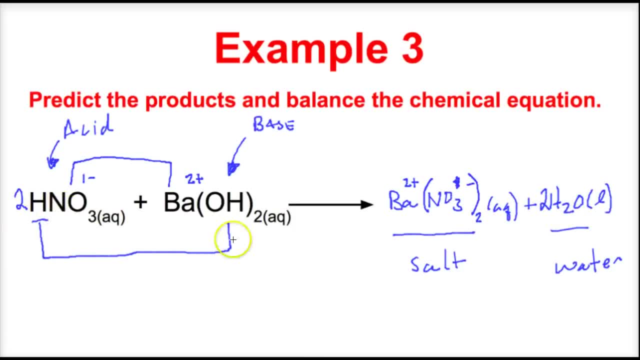 We have 4 hydrogens. on the right We've got 2 nitrogens. on the left here We've got 2 nitrogens. on the right here We've got 6 oxygens here plus the 2 here is 8 oxygens. 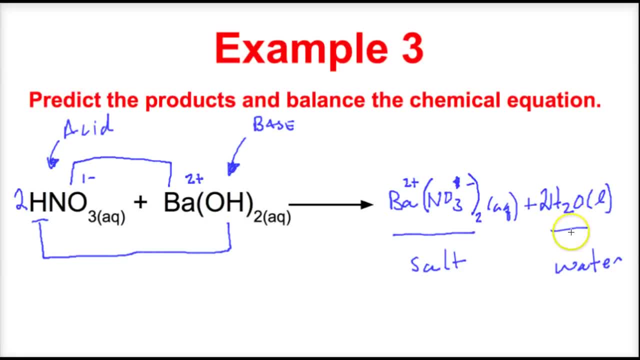 We have 2 times 3 is 6 oxygens, plus the 2 here is 8 oxygens. Those are balanced. And let's see, Last but not least, we've got 1 barium here and 1 barium here. 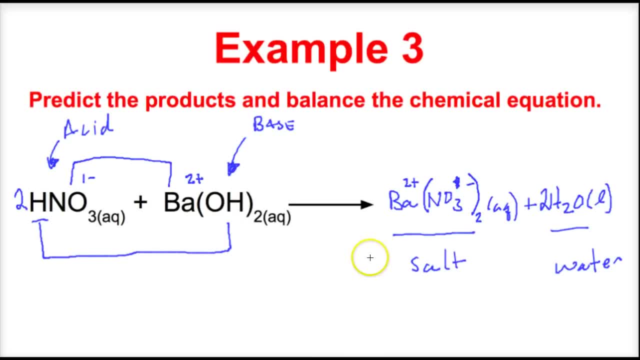 so our chemical equation is balanced. So that's neutralization reactions and I hope this was helpful. 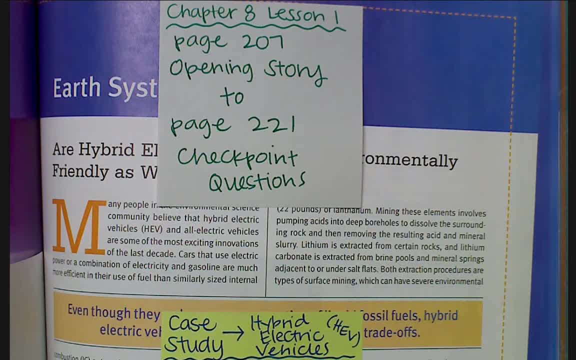 Hey guys, welcome to Chapter 8, Lesson 1.. We're going to start on Chapter 8, Earth Systems. The reading assignment today is on our first sticky note. It's page 207 here on the opening story about hybrid electric vehicles.